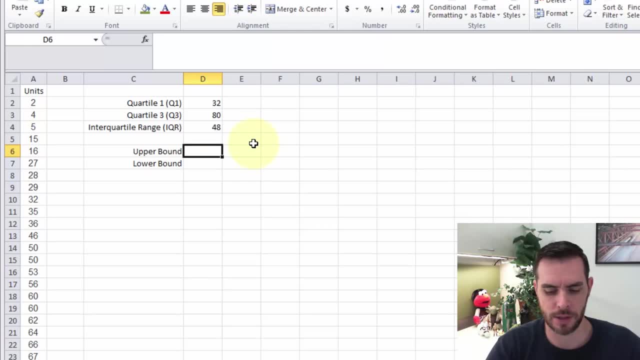 and so now we'll need to solve for the upper bound, and for that we'll say: equals the third quartile plus open parenthesis, 1.5 times the IQR, close parenthesis. Now we'll press enter and that is our upper bound. Now let's calculate for the lower bound and say equals. 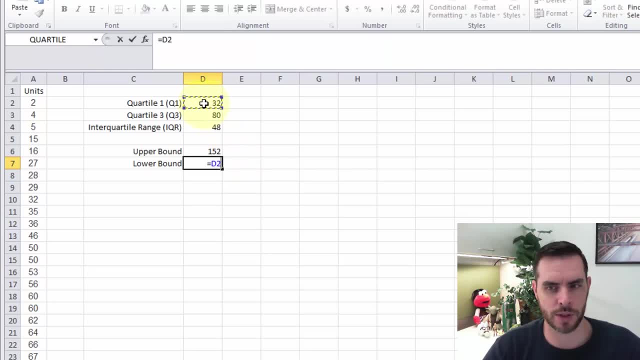 first quartile, minus open parenthesis, 1.5 times the IQR and close parenthesis, and we'll press enter and that's our lower bound. Now we have the range. Anything outside of this range is going to be an outlier. So let's go ahead and run a formula that's going to compare this number to these numbers and we'll 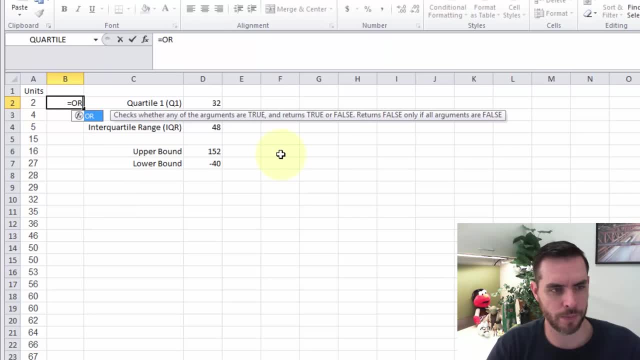 go ahead and say equals or open parenthesis. Then we'll give it some logical comparisons. We'll say A2 greater than 152, or our upper bound comma A2 lesser than our lower bound. close parenthesis. Press enter. So this is saying false. This is not true. So we're going to go ahead and do the same thing over and over again. 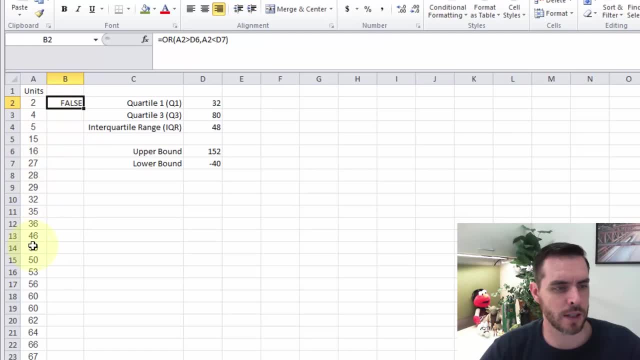 This is not an outlier. Now, to run the rest of these in a quicker fashion, let's go ahead and add some dollar signs to the D6 and D7 parts of the φ quienes formula. Put a dollar sign before the D, Another dollar sign before the 6. Then do. 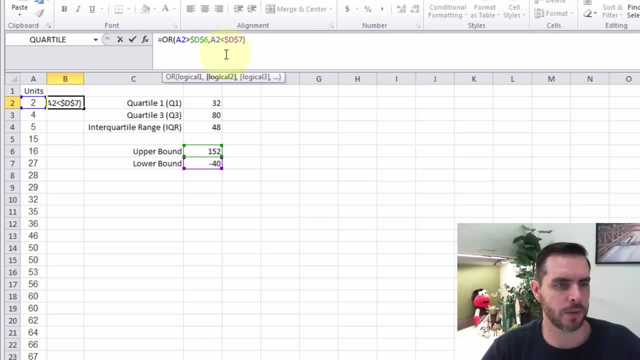 the same thing for D7.. and now we click and drag, it'll always maintain that position, whereas the A2 will be relative to where we're dragging, dragging. So we'll press Enter. and now let's click back on our formula and we'll click. 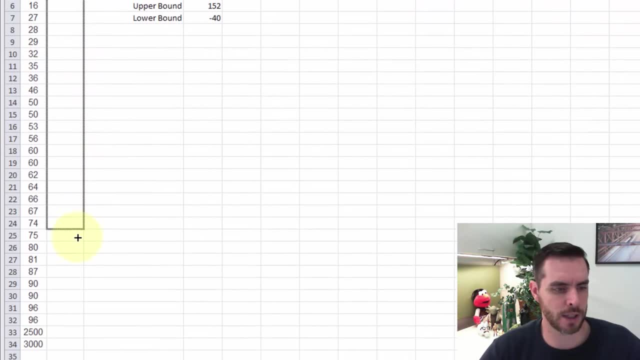 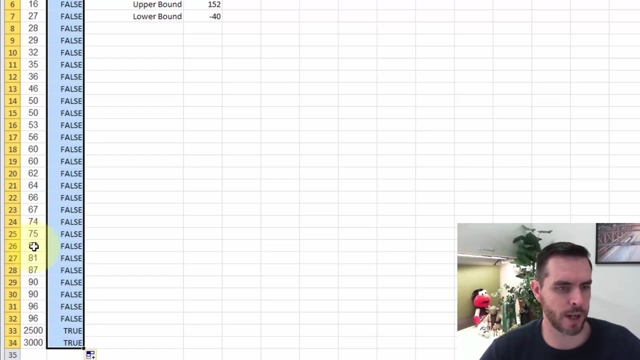 and drag this little handle on the bottom right to continue filling down this formula and release. So now we'll see all these false because they're all within that range that we gave it, except for these last two big ones. It's giving us a true because they're greater.